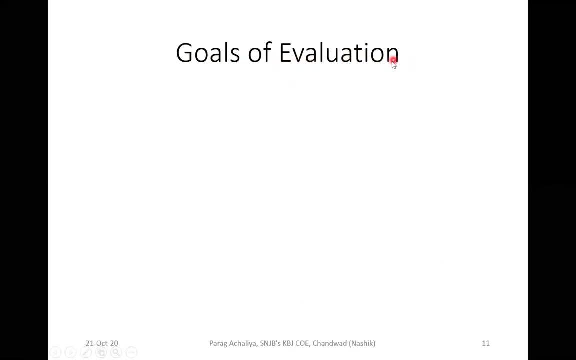 is the need of testing? What is the need of evaluation of any of the system? Evaluation has three main goals. Number one: to assess extent and accessibility of system functionalities. In this point, or the first goal of evaluation will be to check whether the system is accessible. 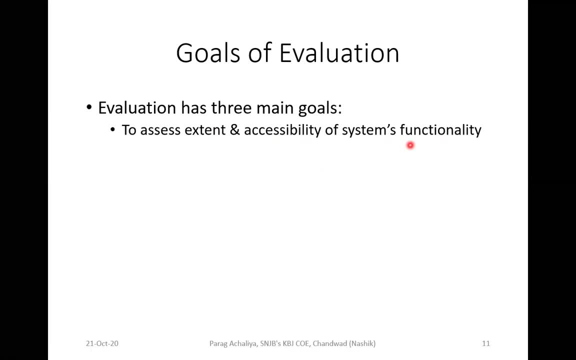 or not, or to check how much your system is accessible. up to what extent your system is accessible? For example, if the system states that it has five modules, then you need to check whether all the five modules will be working or not. Or you are going to check at what extent each 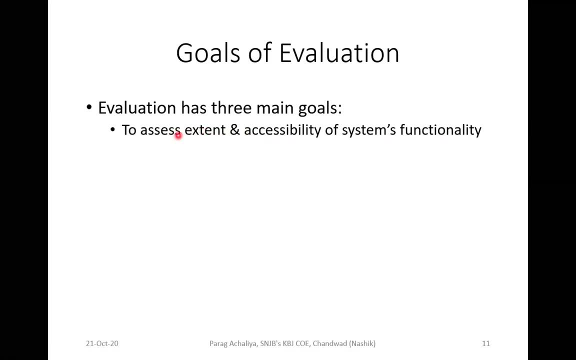 and every module is working. This is what the extent is, And accessibility means whether each and every module is accessible or not, Whether each and every function of the system is accessible or not. that needs to be checked. That is the goal number one of your evaluation. 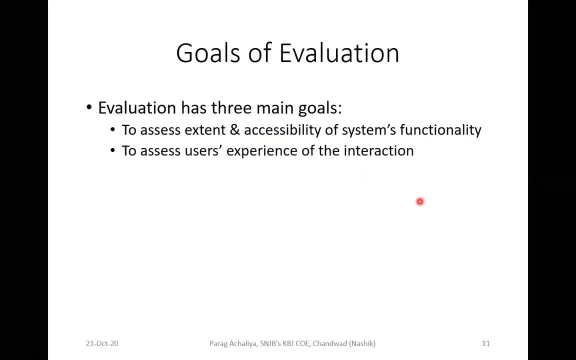 Then second goal states that another goal of evaluation is to assess user's experience of the interaction. What you need to do is you need to assess user's experience of interaction, Whether user is interacting with the system or not. If the user is interacting, then how? 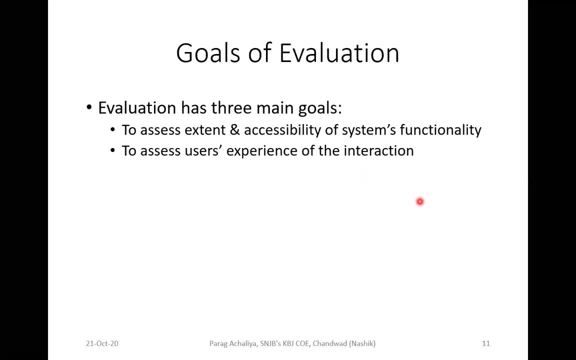 his experience, his or her experience is That needs to be assessed. So, for that purpose, generally, if you observe, Whenever you do your evaluation, you need to assess the user's experience. That is what you need to do. If you do your evaluation, then you need to assess the user's. 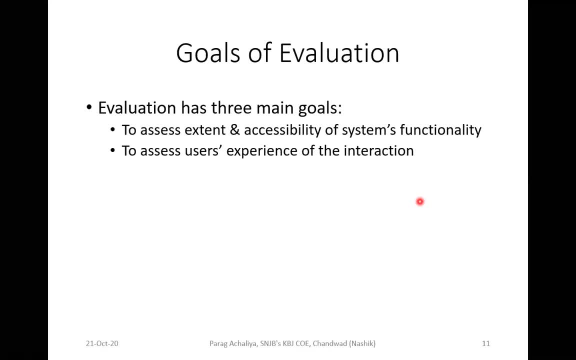 anything online, you generally ask for giving the feedback or rating. so what exactly that feedback or rating is? it is nothing, but they are assessing your experience on the basis of your interaction with them application or with their system. they usually ask you your feedback or they ask you to give the rating for. 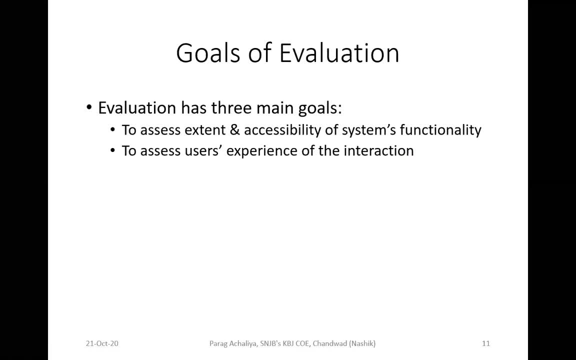 their product or their application or their software. so what exactly that feedback is? it is nothing but to assess the users experience. and third goal is to identify any specific problems with the system. yes, it is one of the important goal. that why there is a need of evaluation to 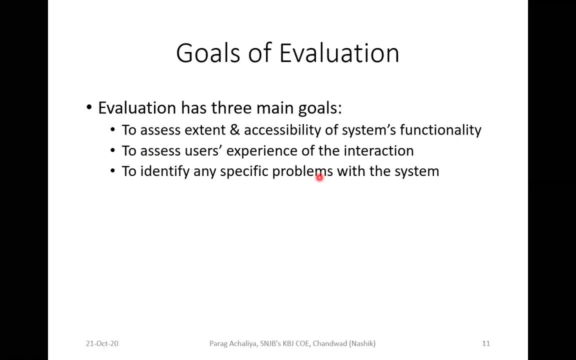 identity to check whether is there any problem in the system or not. if there is any problem, then those problem should be overcome. for that purpose there should be the evaluation of the system. in that case we can call evaluation as your testing. for the third goal, the evaluation word can be treated as the. 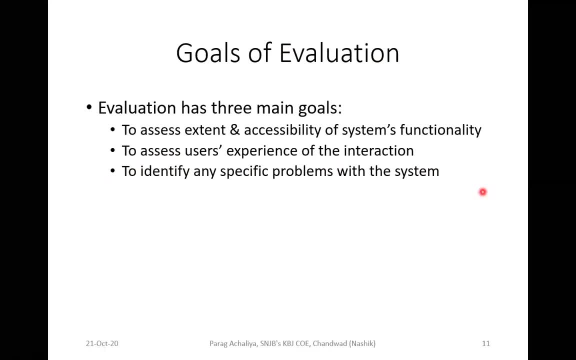 testing of the system. so what exactly the testing means? to identify any specific problem with the system. these are the three main goals of your evaluation every evaluation should carry out for these three reasons. just consider the example of any product. I'm not talking about your software application or web application. just consider any product you can consider. 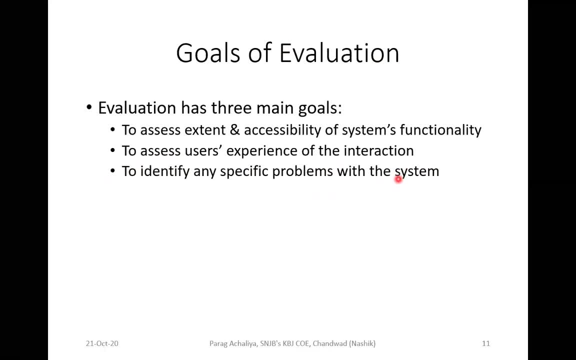 any car, any building, any electronics device, any furniture item, anything, anything you- you can consider the pen, or you can consider your waterboxd depend type, your definition based evaluation or three bottle, anything. you consider any product you are going to evaluate that product. why to evaluate? to check these three activities: how much that product is accessible? what is the user's experience? 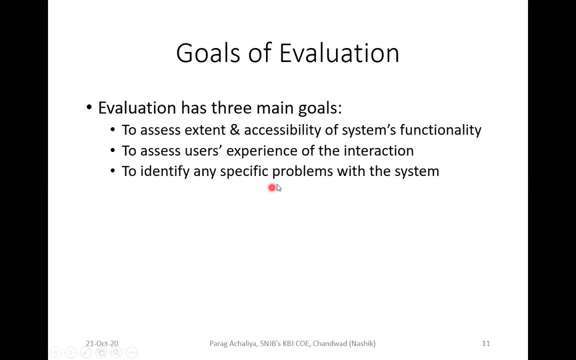 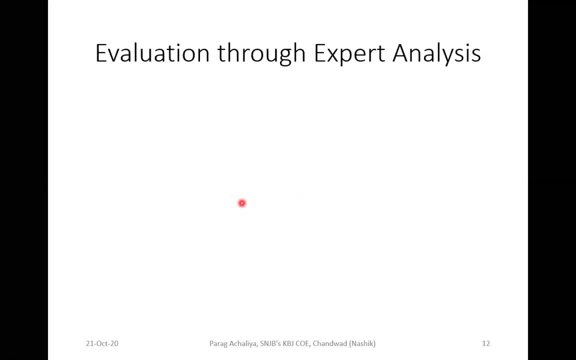 with that product and whether there are any problems with that product or not. these are the three main goals that every evaluation should address. so the evaluation can be done in multiple ways, or evaluation can be done in different ways, out of which the first one will be your. 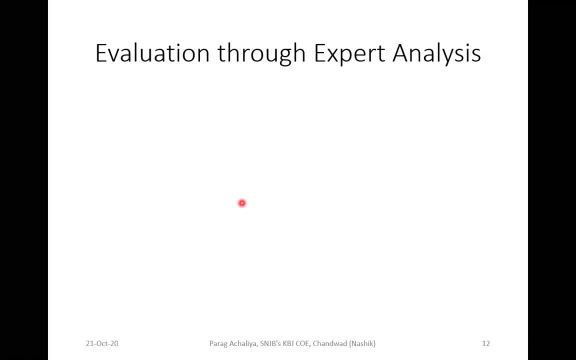 evaluation through expert analysis. the name itself suggests that this type of evaluation can be done by the analysis by the expert. any of the expert will going to analyze your system without executing the system. evaluation should occur throughout the design process. yes, very true. this is very correct that every evaluation activity 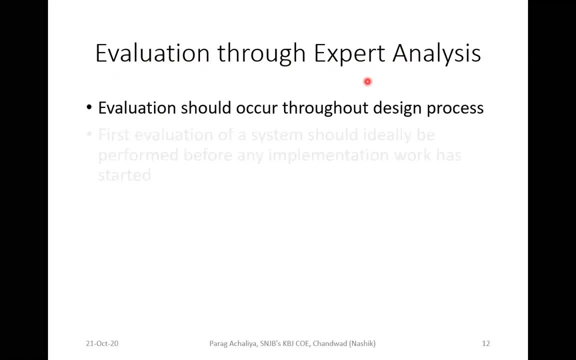 should be done in multiple ways, or evaluation can be done in different ways, out of which the should be carried out throughout your design process. first evaluation of a system should ideally be performed before any implementation work has started. yes, there are two different phases of your software development life cycle. first one is your system design and second one 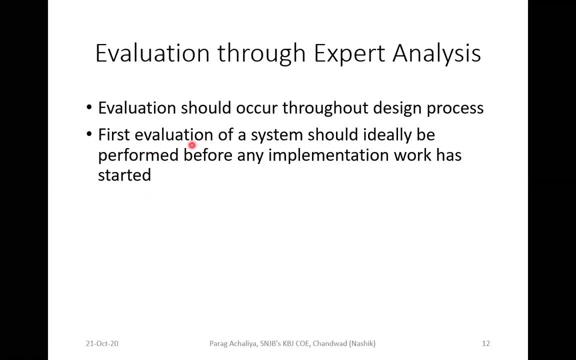 will be your system development, so the first evaluation of the system should be carried out before the implementation work or before your development. that means, ideally, during your design process. if the design itself can be evaluated, expensive mistakes can be avoided, since the design can be altered prior to any major resource commitments. yes, this is the reason why. 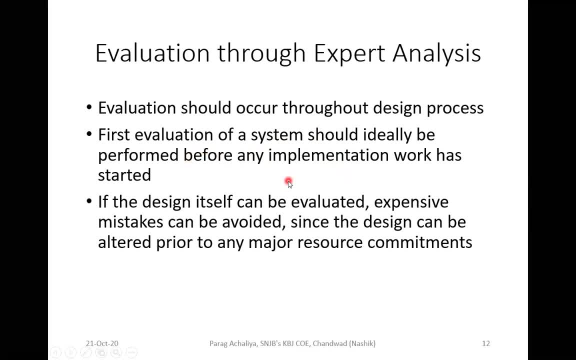 you should do the evaluation before your implementation, or why you should do the evaluation while your design process? because when you evaluate the system at the design phase, you can avoid the expensive mistakes. expensive means this expensive meaning will be the error that can cause very big loss is nothing but your expensive. 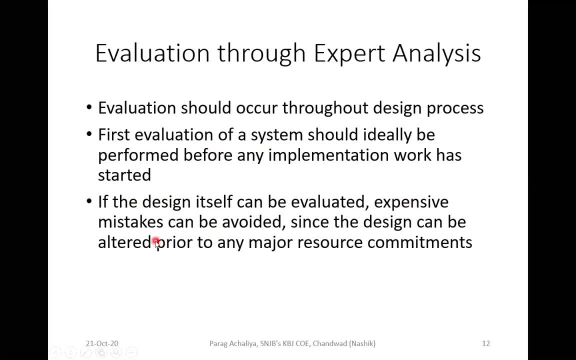 mistake. so in that case those kind of expensive mistakes can be avoided if you evaluate the system during your design phase. it can be expensive to carry out user testing at regular intervals during the design process. yes, that can be your. what expensive activity while you are going to. 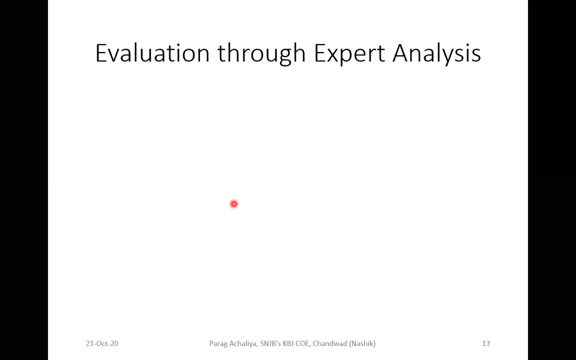 have the testing activity in your design process. there are total four approaches to expert analysis. number one: cognitive walkthrough, heuristic evaluation, use of models and use of previous works. so when you are talking about expert analysis, you consider that the expert will have n number of year of experience in that field. when you call anyone as an expert, 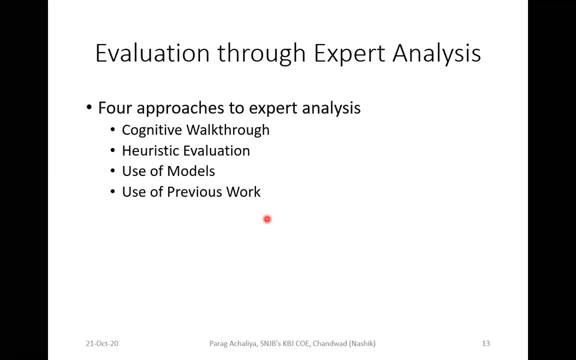 you will call him or her as expert only when that candidate or that person have sufficient amount of experience in that field. then only you will call him or her as a expert. so the expert analysis can be done using these four methods. uh, just for the sake, consider the example of use of previous work. means what if you are doing any? 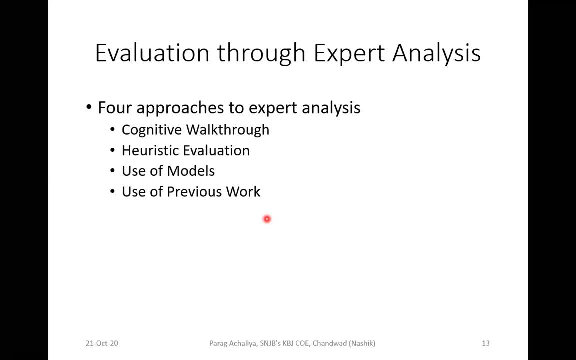 project development. and if the similar project have already been developed, then it will be easy for the expert to give their opinion on that product, because the same project have already been developed and that guide or that person or that expert already know what kind of error can this your project will going to generate. so in that case your expert analysis is very 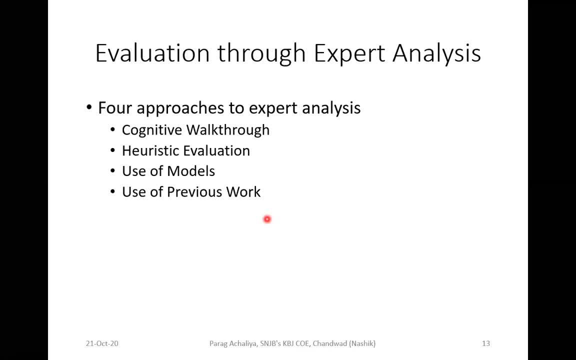 important and expert analysis will be the expert who have very good knowledge in that field. since it's starting of using those four methods, then second type of methodology will be your evaluation through. user participation means what user participation means: actual user will going to participate in the evaluation process. the example of this will be what we can say, that whenever university is. 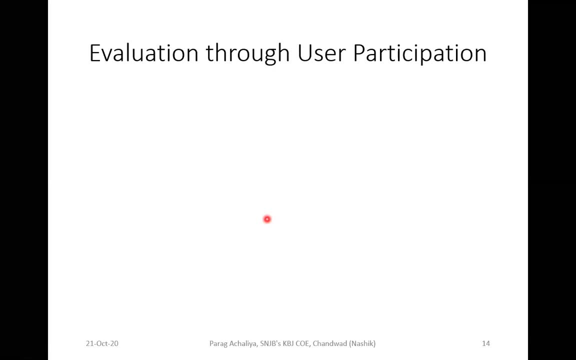 going to launch in a new online portal. they immediately ask you to do your registration on that error or not? so what university is exactly doing? they are evaluating the system through user participation. in that case, you are the user and you are going to use the university portal. 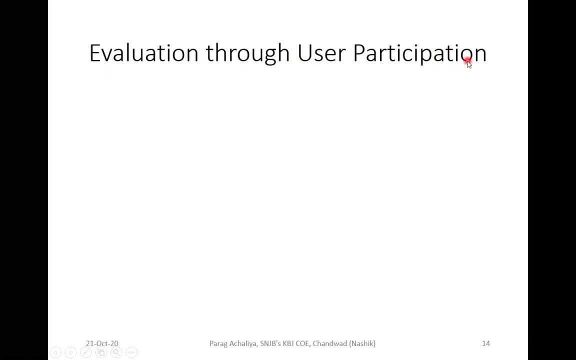 so they are doing the violation by using your experience, whatever problems you are facing, university just collecting those problems and they are trying to find out the solution on those problems. so this is what the activity of your evaluation through user participation, where user is directly, directly involved in the evaluation process. so what are the styles? 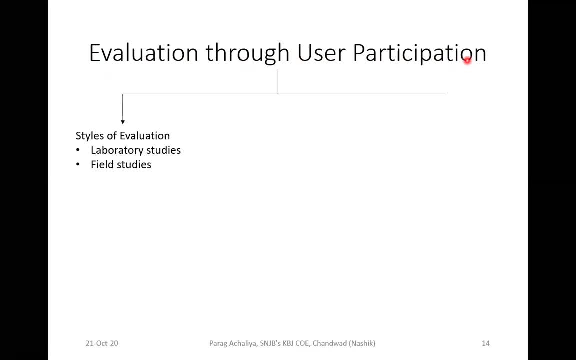 of evaluation. it can be either your laboratory studies or it can be your field studies. laboratory studies means what? whatever you are doing in the lab, that is, your laboratory. and field studies means what- whatever you are going to do on the field, on the live project, on the live field, that 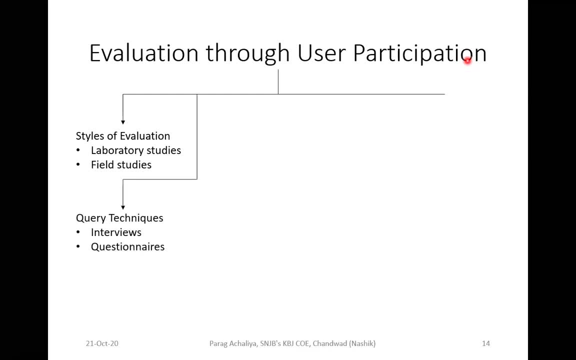 will be your field study. then second will be your query techniques. so query techniques means what you are generating some queries and you are waiting for their answers. so the best example of query technique will be having the interview or questionnaires. interview means what you are going to ask some question and the other person will going to give the answer of those questions. 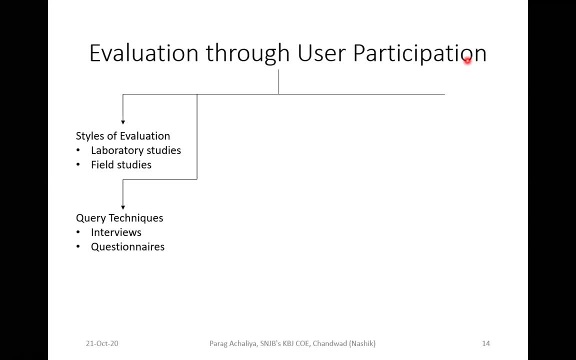 that is nothing but interviewing. and this is the most effective activity of your evaluation: through user participation, because user is going to share his or her experience with you one to one or face to face. that's why query techniques can be either your interview base or it can be your questionnaires. then next one will be your experimental evaluation. means what? 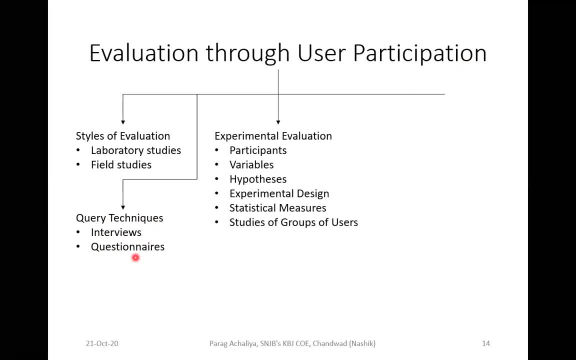 there can be number of questions of participants, variable hypothesis, experimental design, statistical majors, studies of groups of user. these are the part of your experimental evaluation through user participation, because everywhere you can observe, everywhere there are user, user is involved. next is evaluation through monitoring. physiological responses means what? on the basis of eye tracking for usability evaluation. 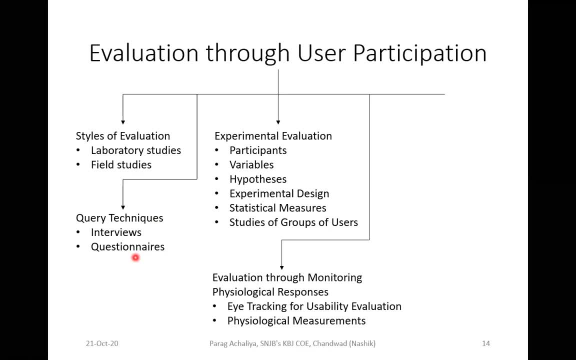 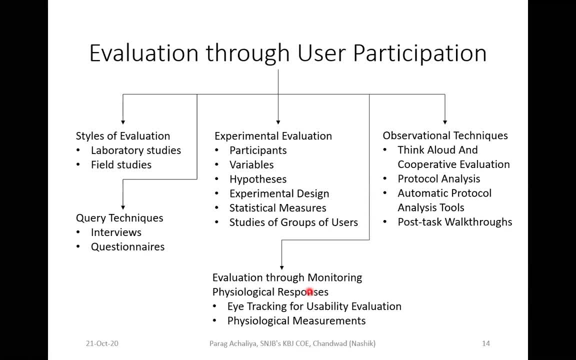 to think aloud or you need to think abroad, and that should be your cooperative evaluation. that means everyone should be cooperatively work on the evaluation process. then next one will be your protocol analysis. you need to analyze the different protocols, whether the evaluation technique is going to follow the protocol or not. that you need to do using your automatic. 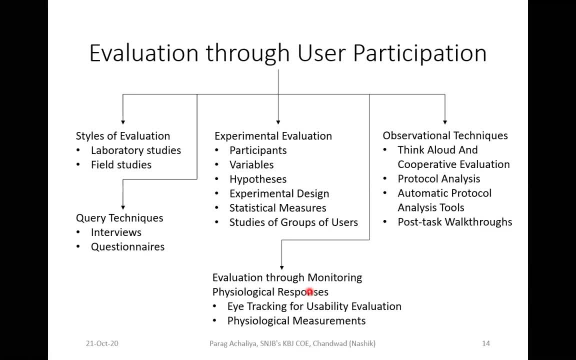 protocol analysis tool. and next one will be your post task walkthrough. means what? after completing the task, what will happen? that is nothing but your post task walkthrough. so this is what you need to do. so this is what you need to do. so this is what you need to do. so this is. 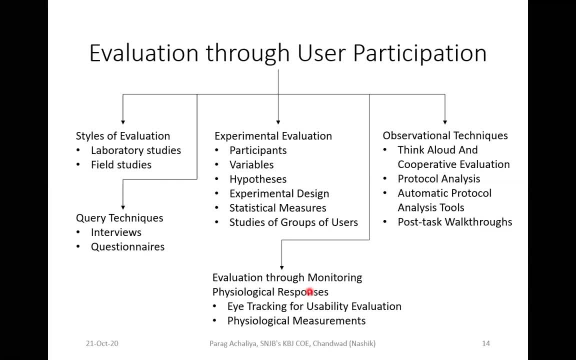 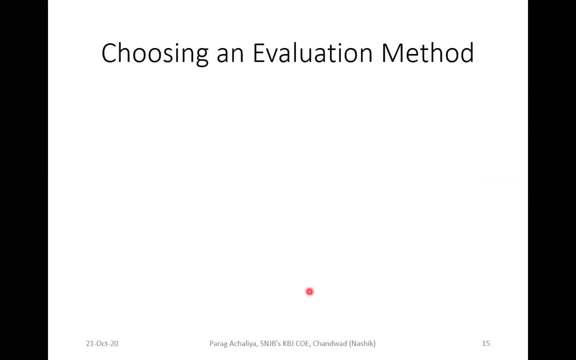 what your evaluation types of our, we can say, categories of evaluation of this system through user participation. so the next question will be which evaluation method you are going to use, or which evaluation method you are going to choose out of those evaluation methods we have already discussed. so which one will you choose? so for that also there are some criteria. if this happened, 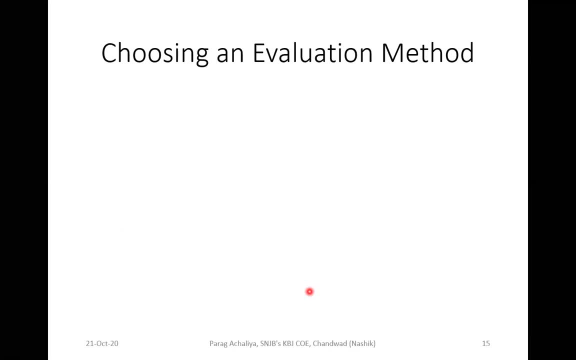 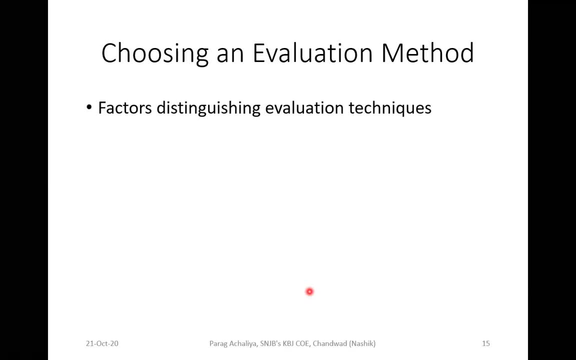 method. so which are those criteria? there are some factors which are going to distinguish various evaluation techniques. which factors? number one: the stage in which- sorry, the stage in cycle at which- evaluation is carried out means where are you doing evaluation, whether it will be in design phase, or it will be in development phase, or it will be in implementation. 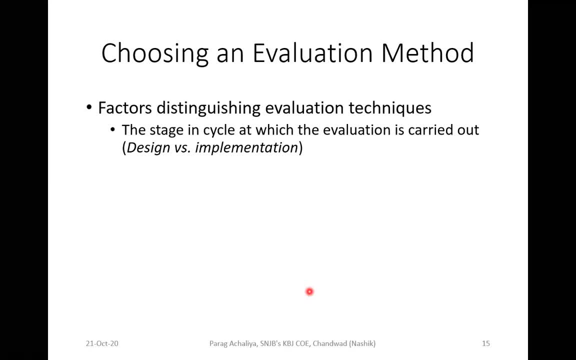 phase. on the basis of this, you are going to decide which evaluation technique should be used then. second one will be: you need to identify the style of evaluation means- whether it is laboratory study or it will be your field study- then the level of subjectivity or objectivity of the technique that 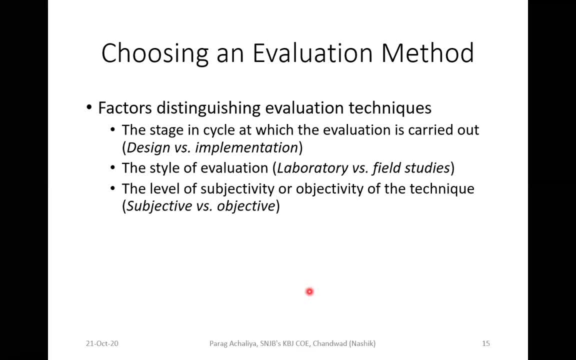 means whether the it is subjective or it is objective. on the basis of this again, your evaluation technique will going to change the type of measures provided. that means you are going to focus on quality or quantity that you need to study or you need to identify the idea. 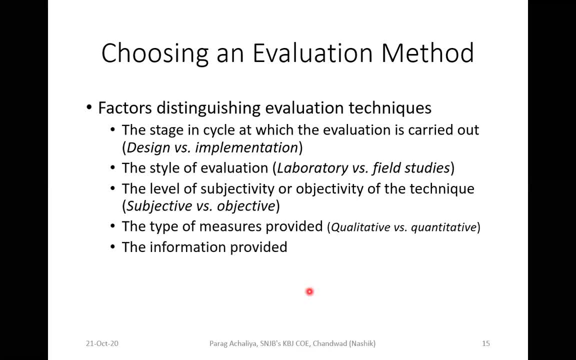 then You are going to select the evaluation sino образом, based upon the provided information or whatever meaning that you are going to receive. based on that, you are going to decide which evaluation method you need to select for a system evaluation. then speed of the response means what. 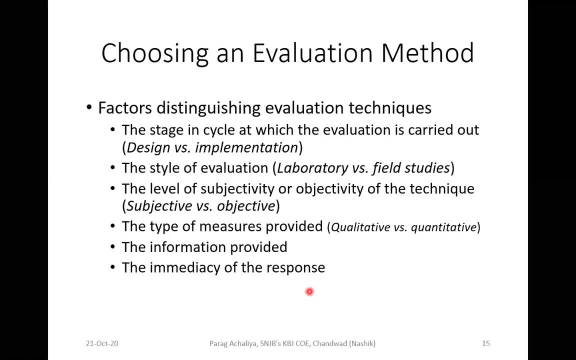 how can you receive the response from the system immediately taste the which isorar y sucroial basis of that. also, you are going to decide which evaluation technique you are going to use. So the response from the other end is also very important factor while considering your 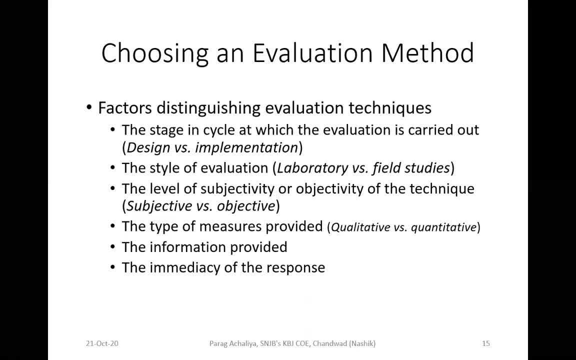 evaluation techniques. Then next is the level of interference implied. how much interference is there applied by the external agency? that is again the factor that will going to focus on evaluation technique. Then the next is how many resources you required, which different resources you required on. 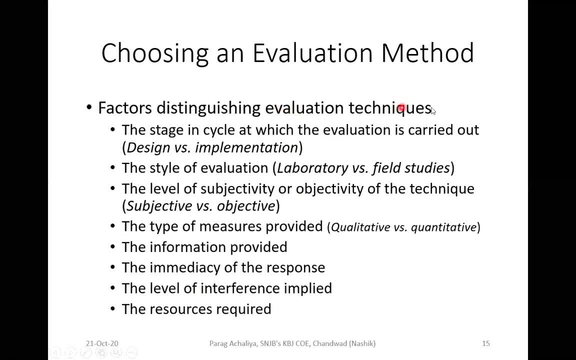 the basis of that also, you are going to select your evaluation technique. Just for example, you do not require any kind of resource for your expert analysis- expert analysis- in this case. you will not require any kind of resources. only you will be requiring one expert and that expert.